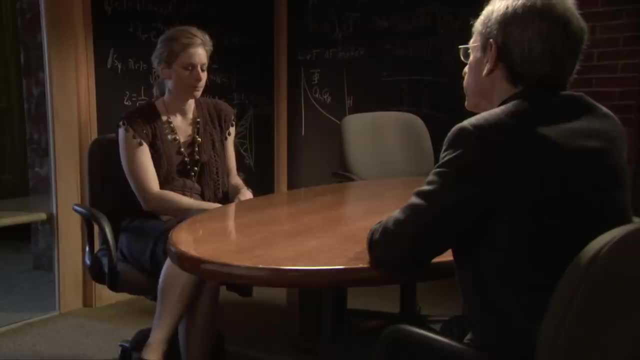 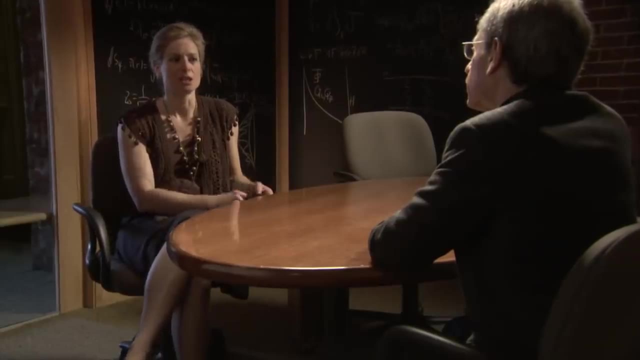 which would be like left, right forward, backward, up down. But one of the best ways to imagine how we should envision extra dimensions was actually done by Edwin A Abbott in the late 19th century in a book called Flatland, And what he said is: if you lived in two dimensions, you would have the 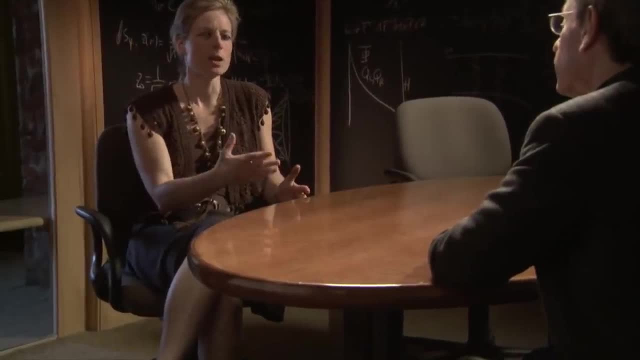 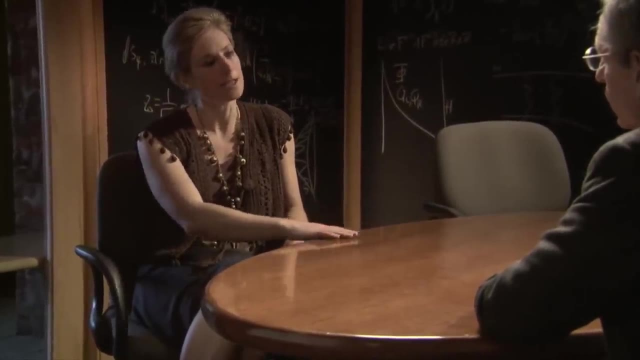 same difficulties picturing and imagining third dimension that we have imagining a fourth spatial dimension or higher dimensions. So what he said is: suppose that there were a creature living on Flatland, say, this tabletop, and how would they see the world? And I mean we know. 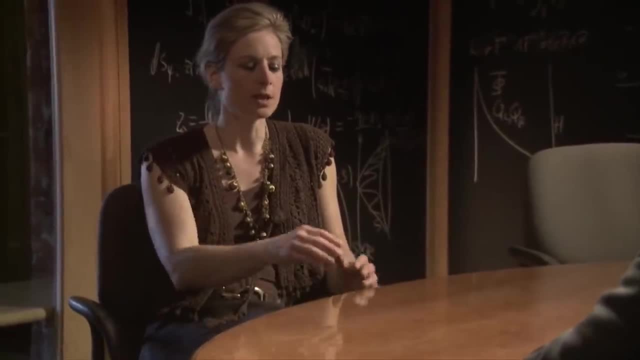 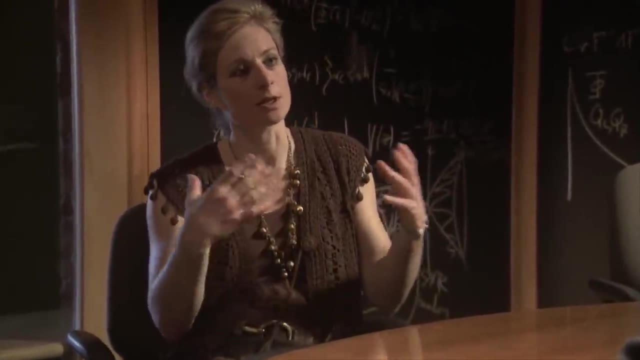 there's a third dimension, but these Flatlanders wouldn't be aware of it. So what would they see? Well, suppose some object like from the third dimension came through. Suppose a sphere came through. A Flatlander would never see the sphere in its entirety. They can't see three dimensions. 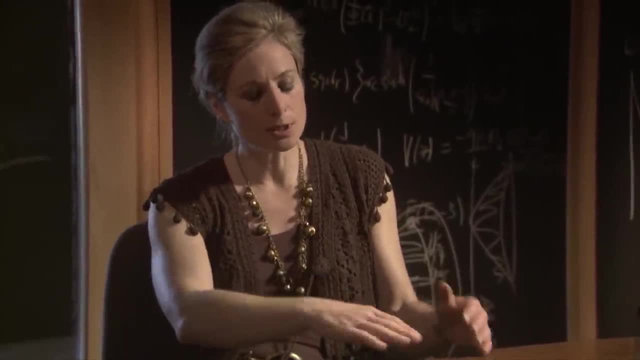 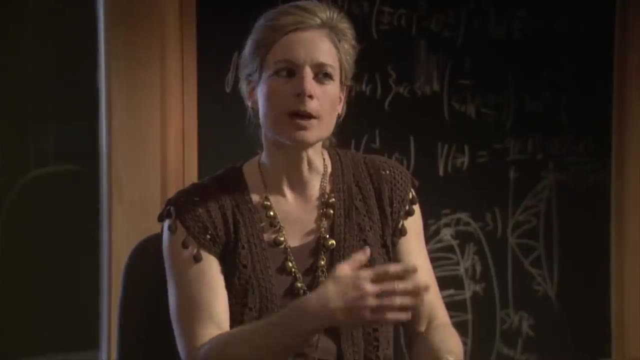 the same way, we can see more than three dimensions. But what they would see is a series of disks that grew in size and then decreased in size as the sphere went through. So they would get all the information, So they would know about third dimension or about this three-dimensional object, even though they 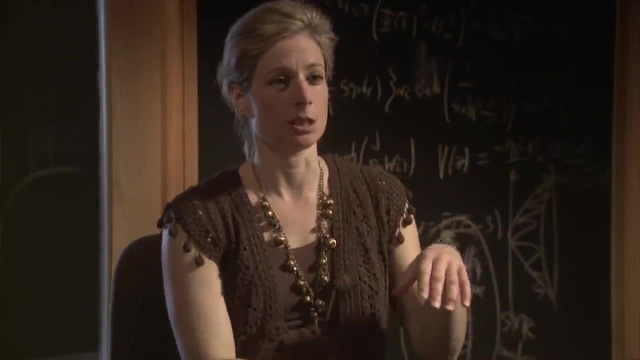 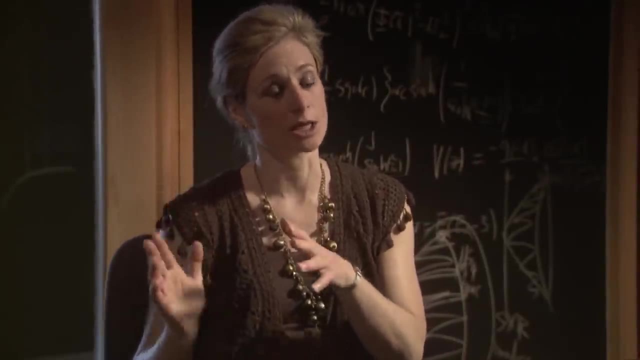 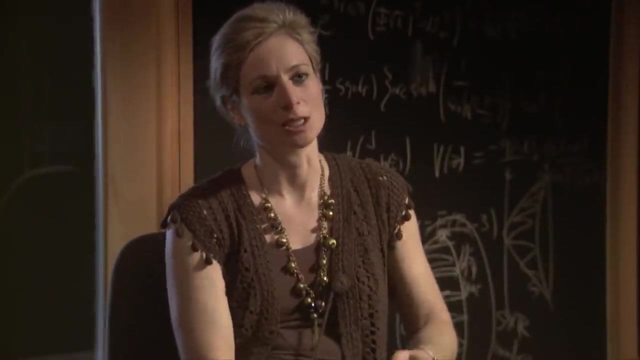 couldn't necessarily reconstruct it in their pictures to see that it was a three-dimensional object. So in the same way, it could be that there are extra dimensions that we don't see directly, But we can see the implications of those, But there could be signs that we could put together to tell that those dimensions exist. 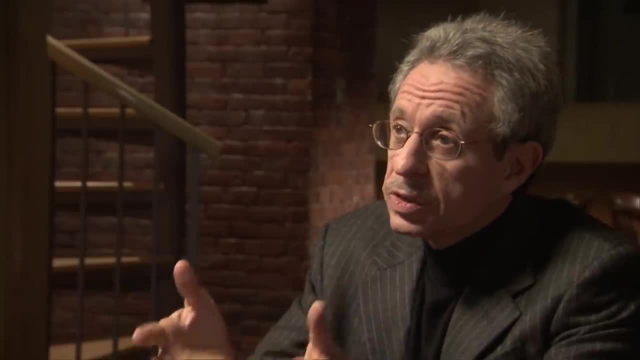 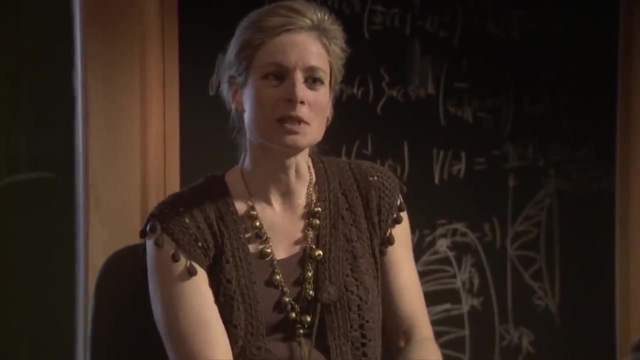 So what are the motivations from physics' point of view? Why does physics seem to have a need for these extra dimensions? Well, some people would say we do have a need. Some people would say we don't. I don't want to overstate it. 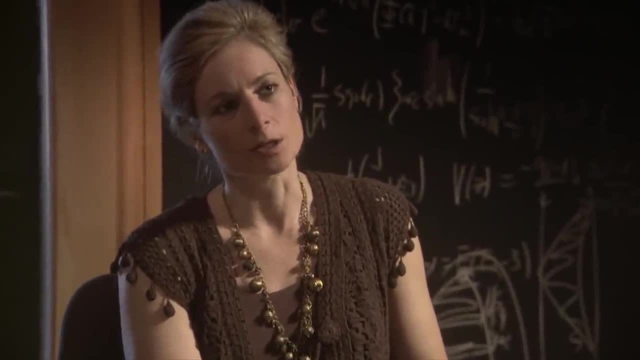 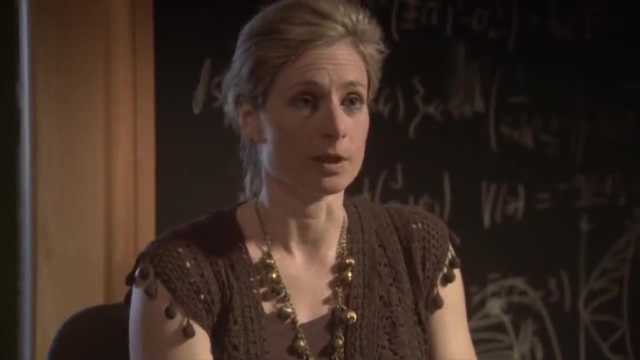 But there are several reasons why we think about extra dimensions. One is a theory called string theory, which is a theory of quantum gravity, or a purported theory of quantum gravity, trying to put together general relativity and quantum mechanics, And the point is that theory doesn't make sense. 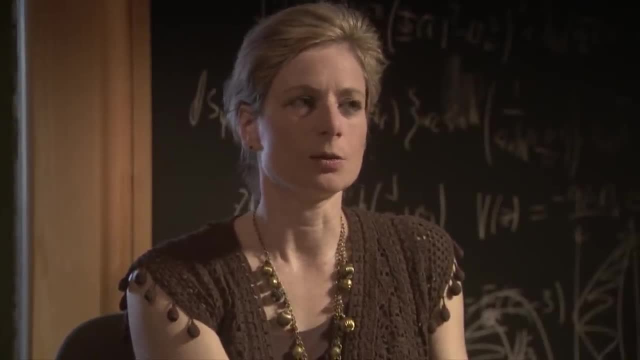 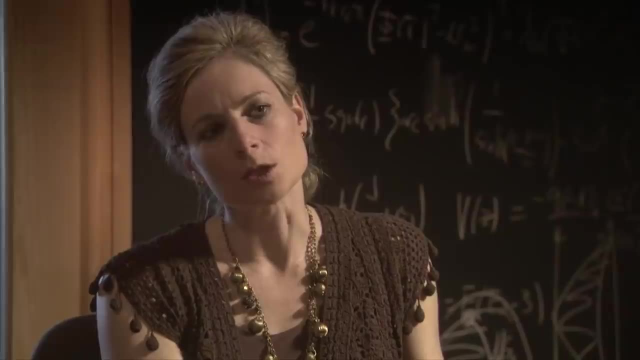 if there are only three dimensions of space, You need extra dimensions. So then, the question for a physicist is: what are the implications of those extra dimensions, and why haven't we seen them? But there are other reasons, too, And one reason that I find very compelling is that there really are. 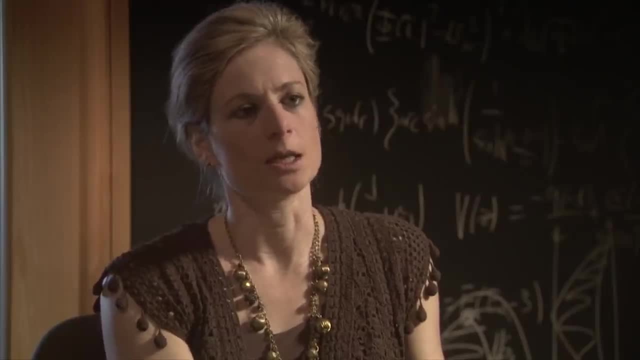 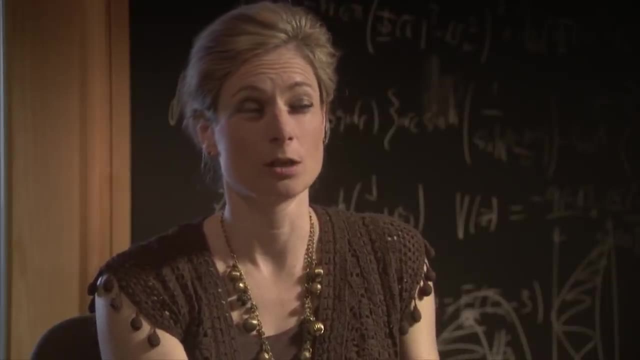 problems in particle physics that are very difficult to address in the context of just three spatial dimensions. The Standard Model of Particle Physics, which describes matter's most basic elements in their interactions, was put together in the 1970s, And there are some outstanding questions. 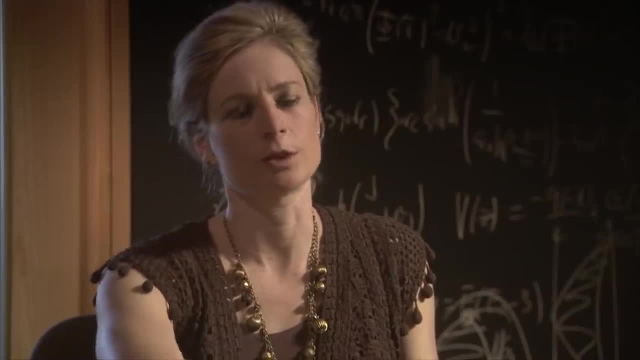 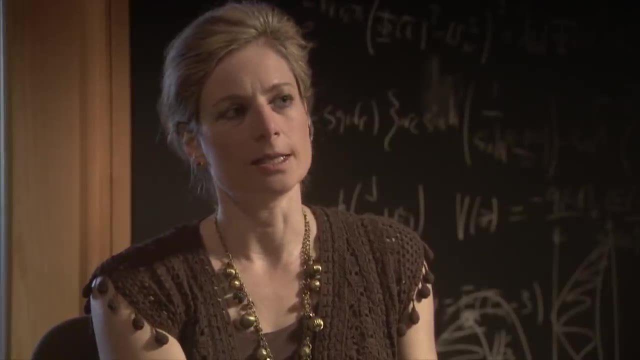 Although the model works beautifully- it makes beautiful predictions, agrees with experiments of a high level of precision- there are some fundamental elements of that theory that we don't understand yet. People have been trying to solve it, as I said, since the 70s and haven't come up with a completely compelling. 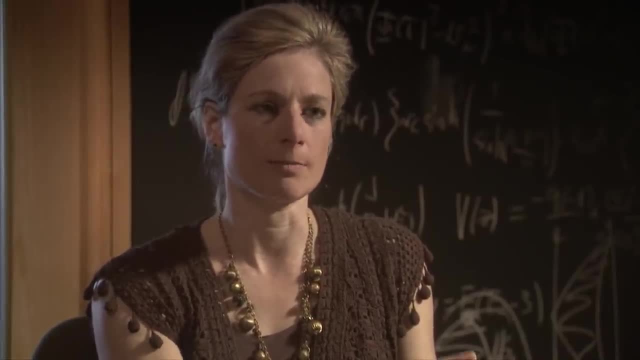 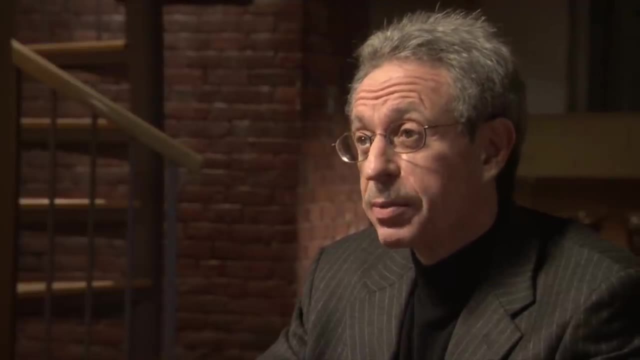 solution, And it seems that if there are extra dimensions of space it might be easier to find ways to address them. And also in the Standard Model of Particle Physics we have so many different parameters that have to be entered by hand that can't just fall out of the- what? are they 26 or some large numbers? 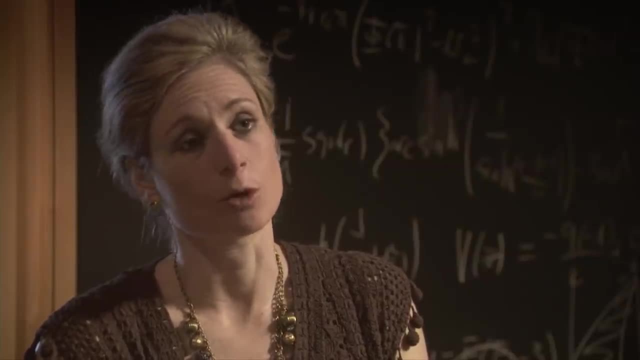 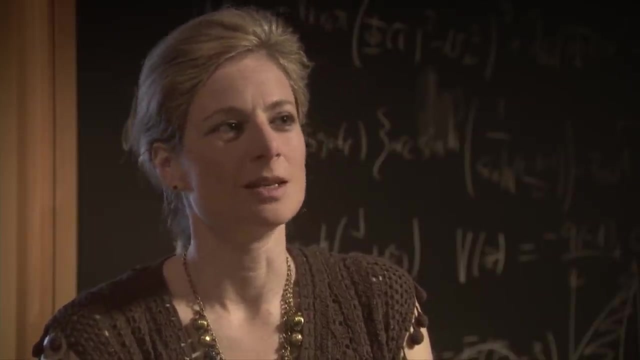 Well, there are a lot of parameters in the Standard Model, namely masses of particles, charges, etc. And there are ways of trying to address them. Well, there are ways of trying to address them in the context of three-dimensional space. But again, if I showed you one of these examples, you would say that looks pretty complicated. 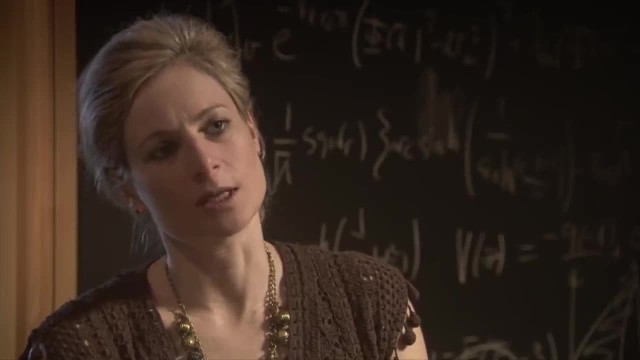 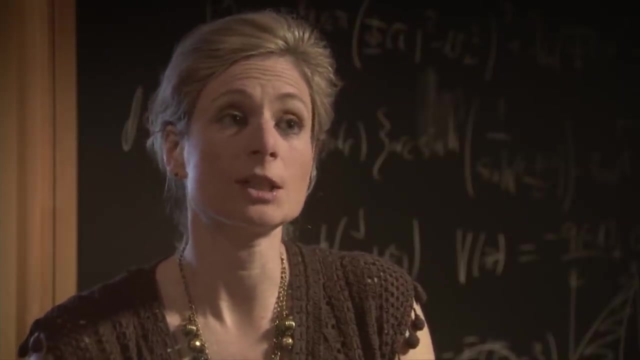 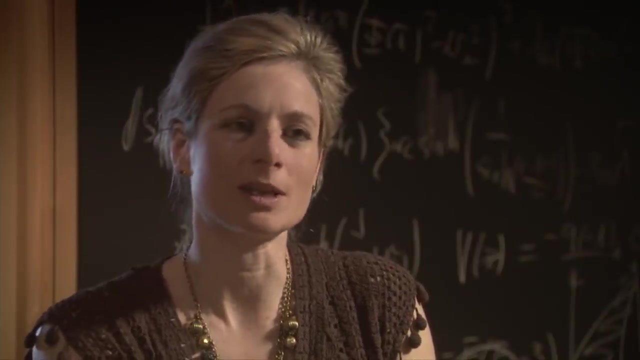 And so another possibility is that we can have extra dimensions and try to address it there, And we don't know the answers, We don't know that those problems will be solved. But it's a new forum and there's a lot of new ideas. I should say that, even if these ideas about extra dimensions turn out not to be right, it turns out that they've given rise to new ways of thinking about even three dimensions. So there really are new ideas that have come about. 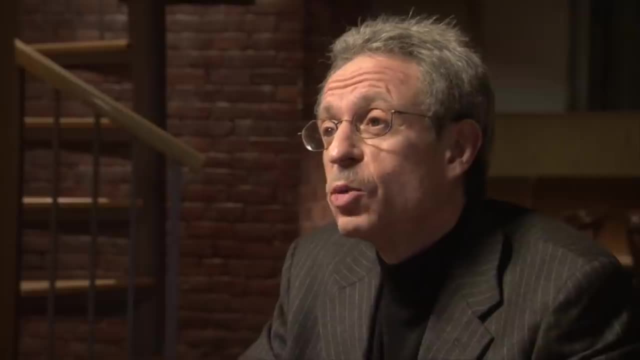 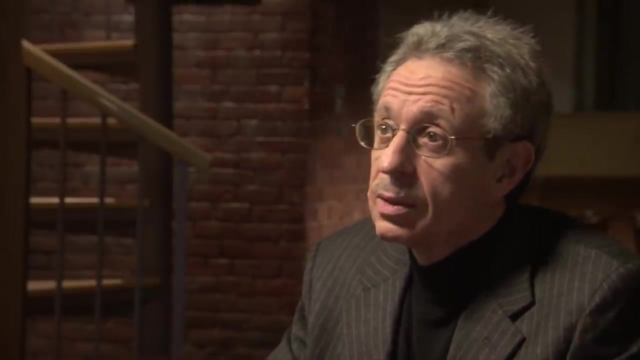 I think that's terrific. That's the most important. I think that's part of new ideas. It's not necessarily that they have to be right, but that they force us to rethink our conception of everything else that we're doing, Although we do prefer if they're right. 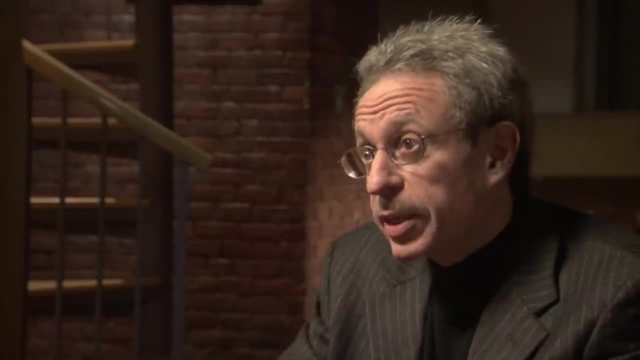 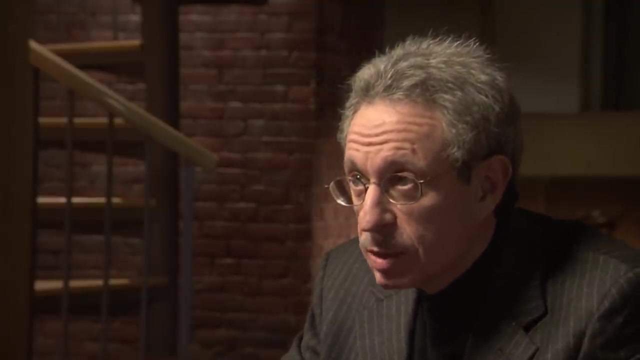 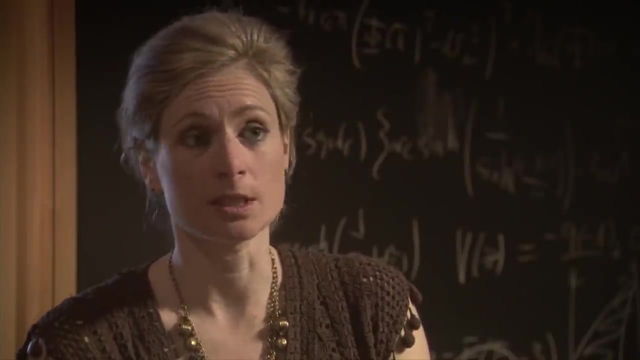 Right, Of course. Let's talk about some of these extra dimensions. What do they look like? I know the word is compactification, which means they're extremely small. they're curled up. How can we understand these extra dimensions? Well, that's one way of, but actually another possibility is that they're very curved or warped. the way Einstein taught us can be true in present-day science. 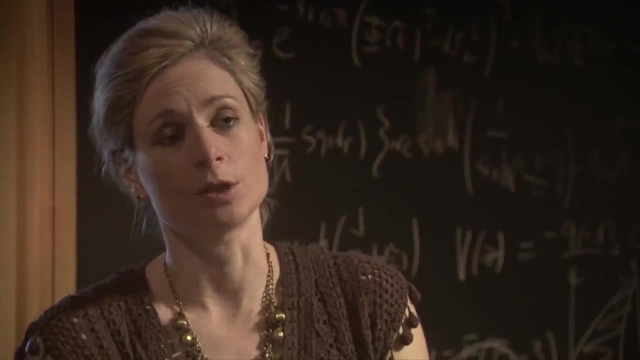 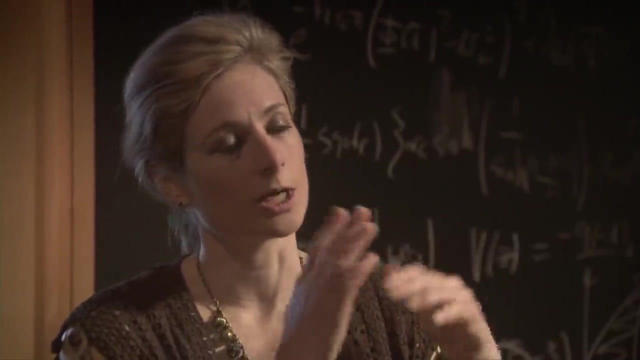 Mm-hmm, Mm-hmm, Mm-hmm. They have a presence of energy And the implications of the extra dimensions can be very different depending on whether they're hidden because they're very tiny, or hidden because they're very warped. 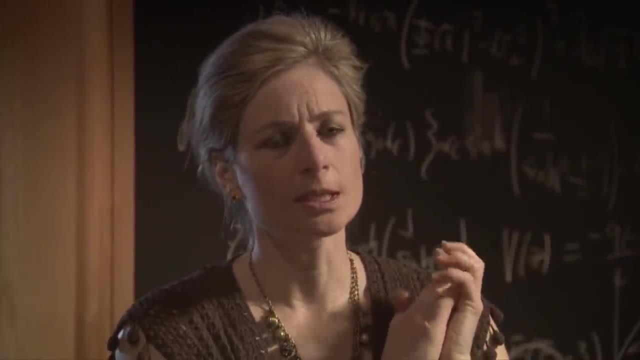 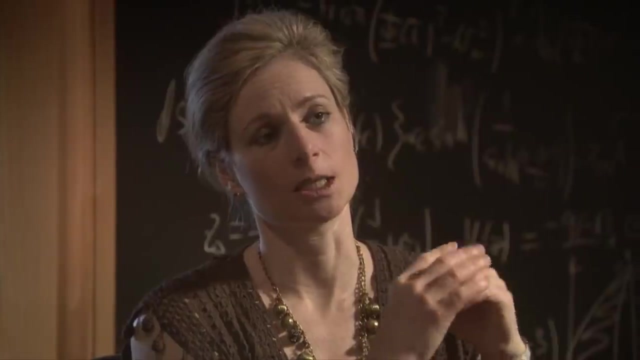 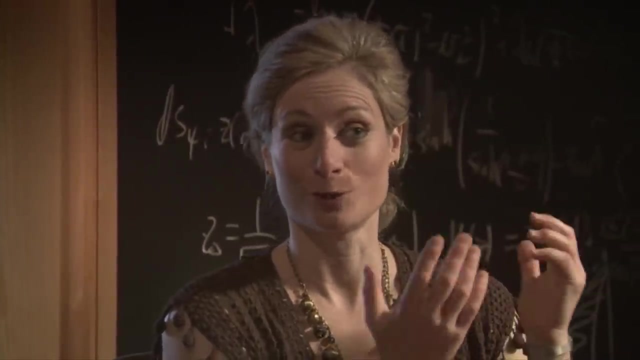 Wow. So basically soon after the idea of extra dimensions was introduced in the context of physics, And so basically in the 1920s, people started thinking about this idea that you could have very tiny dimensions, And the idea is rather intuitive. which is something is really small? you don't see it? 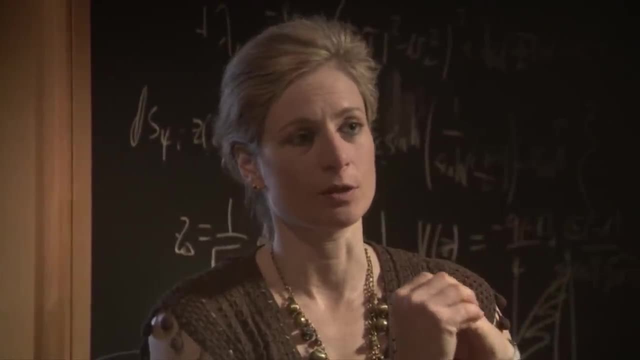 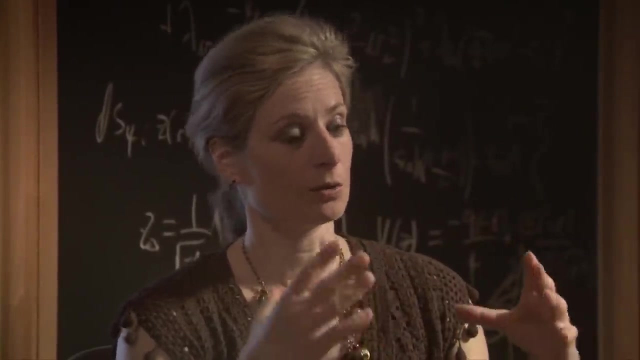 Yeah, And that's basically what's going on, perhaps with extra dimensions of the universe, dimensions of the universe. However, as I said a moment ago, it could be also that space-time is really dramatically warped so that we only really experience one region of space and 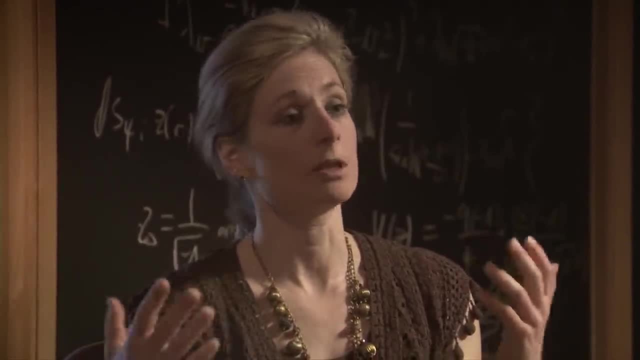 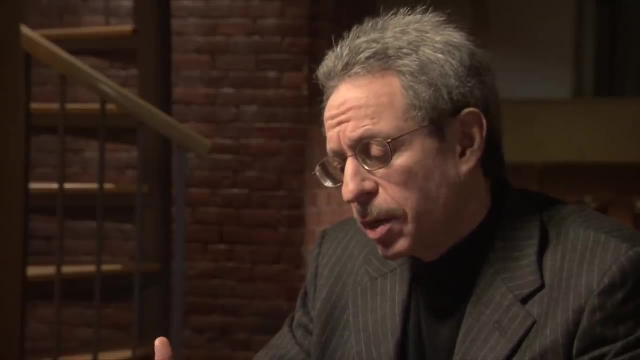 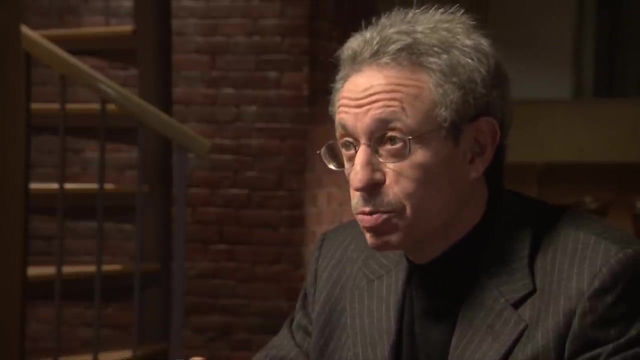 other regions of space have less influence on us, And that could be another way that extra dimensions could be hidden. Let's talk about gravity in the context of extra dimensions, because gravity seems to be the one part of reality that can communicate through extra dimensions, because it's related. 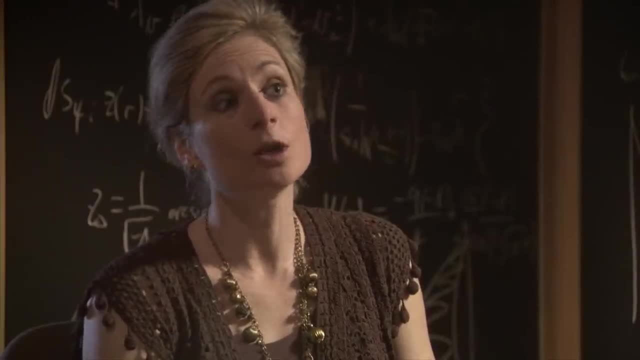 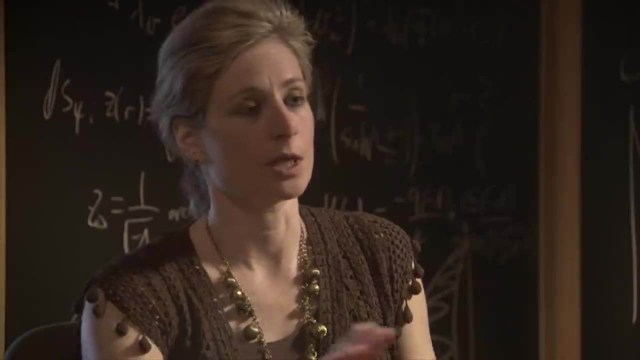 to space-time itself. I should say gravity is the one part we know should be intimately connected to all of space-time. There could be other particles, There could be other forces that communicate through extra dimensions, But gravity is one that we know has to be there. 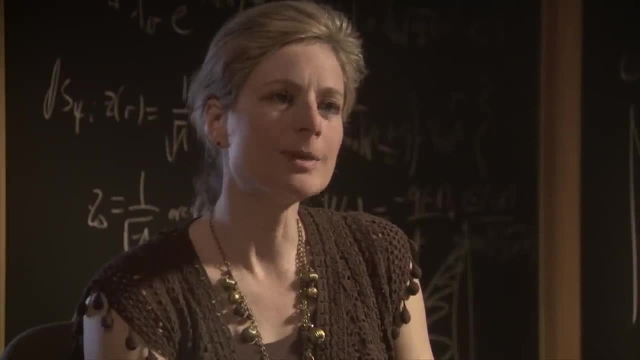 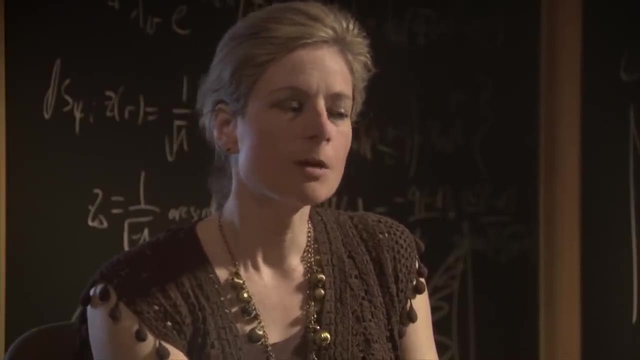 And it has to be there. because It has to be there, for…basically, Einstein taught us that it has to be there in some sense, because one thing is that gravity is connected to the geometry of space-time, But another way of understanding it is that gravity is something that interacts with energy. If 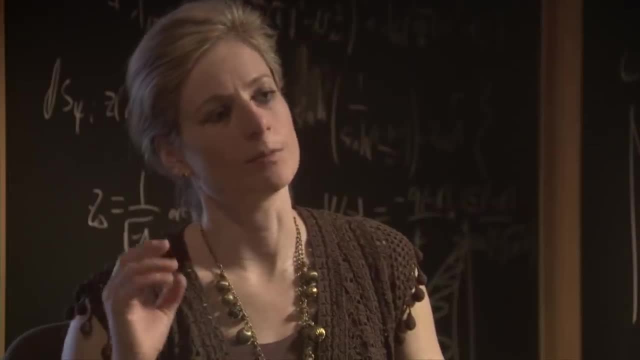 you have energy at a certain point in time. you have energy at a certain point in time. If you have a magnetic object, it creates a gravitational field. If something is moving through a gravitational field and has mass or energy, it experiences gravity And it. 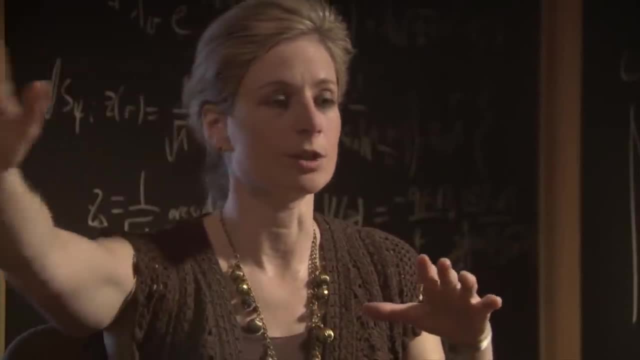 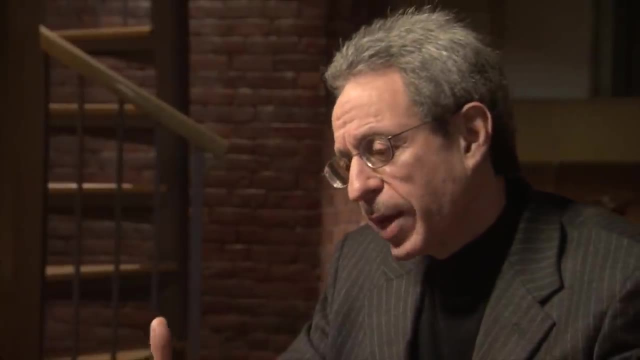 better be true that that's true anywhere, That if you have energy in any region of space, whether it's here or off in an extra dimension, it still should experience gravity. And the fact that it's an extra dimension we haven't seen it doesn't mean that the 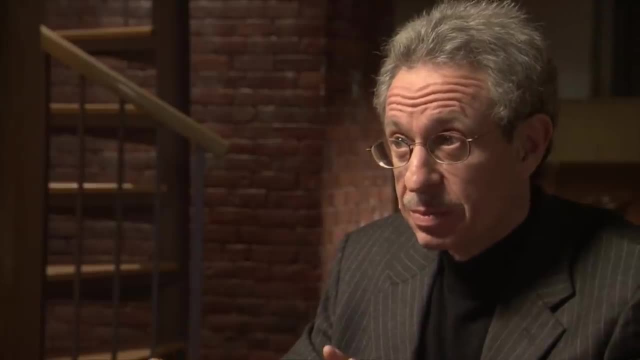 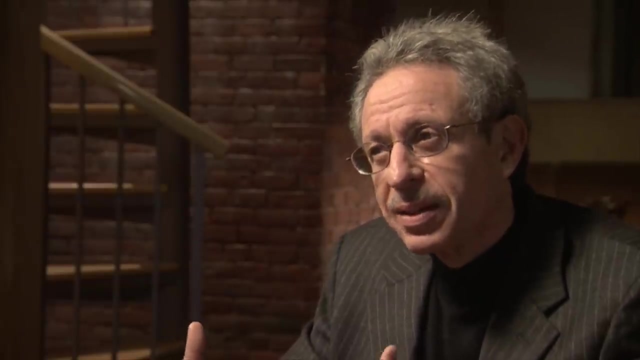 kind of gravity that we're experiencing will…it may be different. I mean the fact that it's a dimension itself. gravity must be similar in that dimension, because since we know so little about it…. Okay, So what we know is the fundamental gravitational theory. Then how we experience. 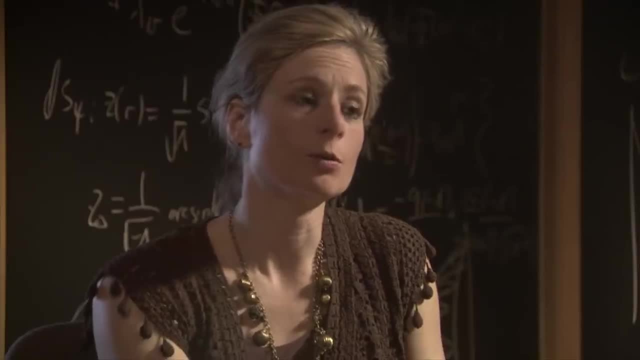 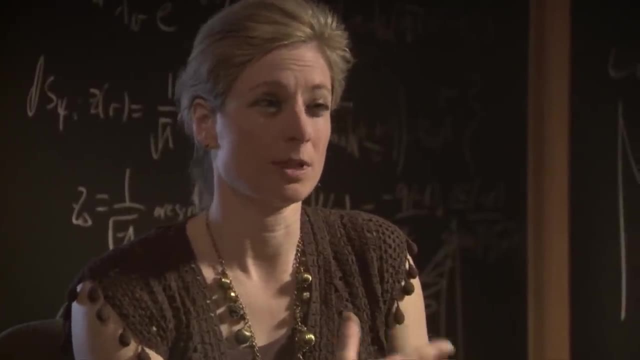 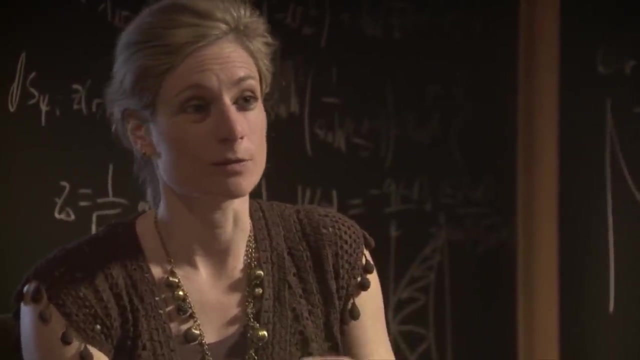 gravity depends on the distribution of matter and energy, which defines which gravitational field is in our environment. So there are many different ways that gravity could be experienced in our world, and that's one of the things that we explore. For example, if you're near a black hole, you experience a very different sort of gravity than if you're. 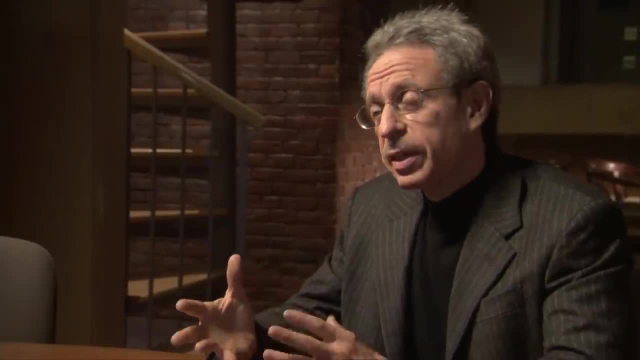 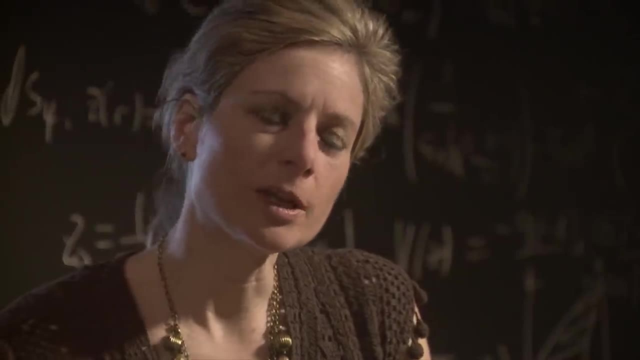 in our environment here, Right? Is that a good analogy to the gravity and extra dimensions to see what happens in black holes, where you have this enormous warping of space-time? There you have the…in the black hole case, you sort of have the warping of time for. 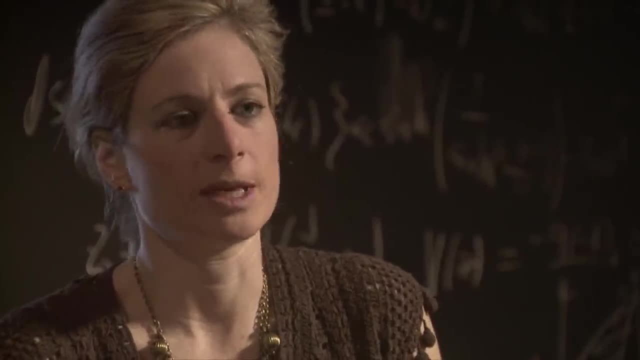 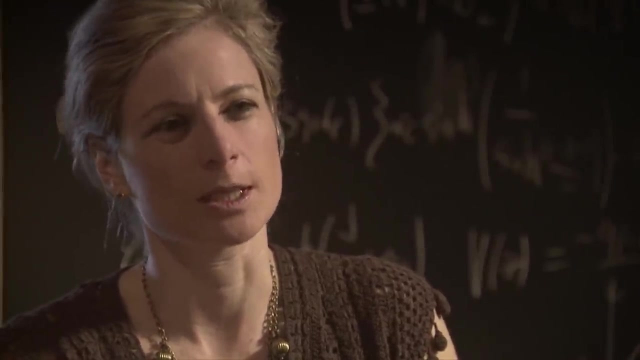 example, Right And in extra dimensions. you could warp space and time, for example. I see, I mean you also get warping in some sense of space, but it works differently in the context of a black hole. But it is a good analogy in some ways. 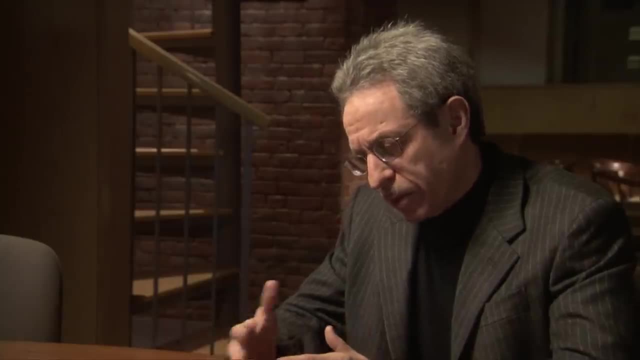 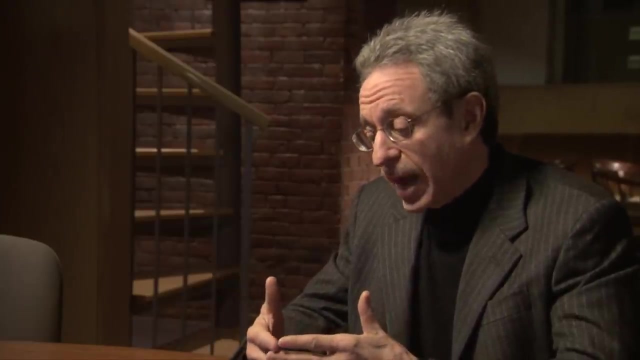 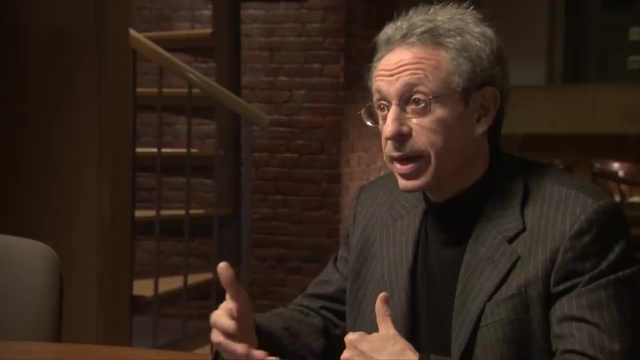 Is there any way that the extra dimensions and the gravity communication between them can help us with what we're seeing? Well, we're seeing a very interesting thing. We're seeing what seems to be a very strange reality where the gravitational power is so much weaker than, for example, electromagnetic. 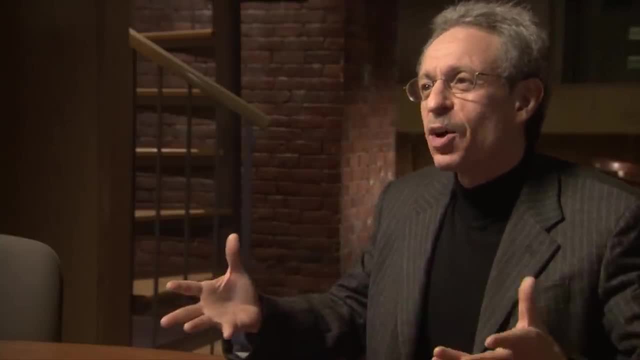 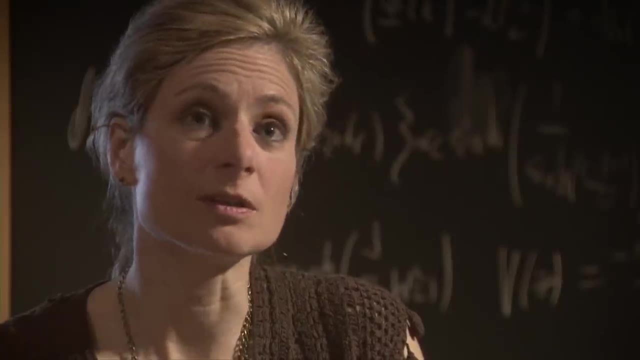 forces. That's right, Like 10 to the 40th. It just seems an odd thing in our world that two of the primary forces have this enormous difference in power. That's right, And it's worse than just a mysterious question, because if you take the principles, 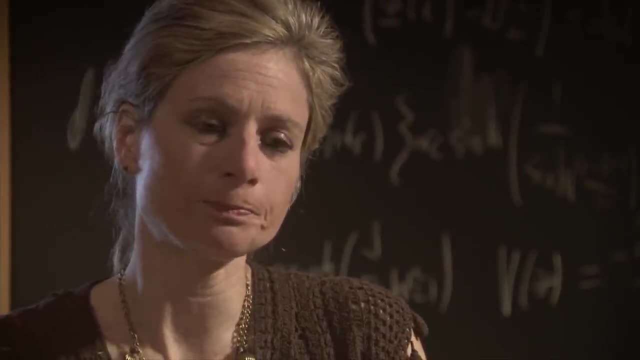 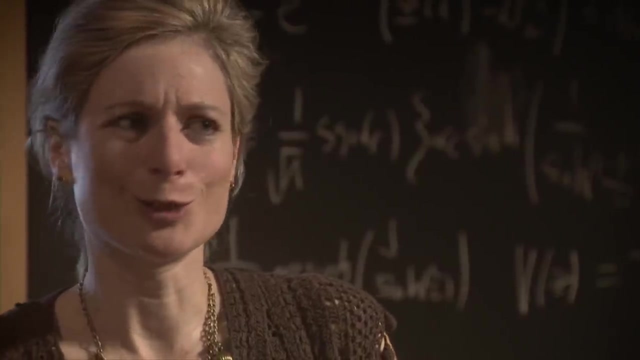 we believe are true—namely quantum mechanics and special relativity—and put them together and try to predict how these forces should be related. it would be much more natural for them to be of the same order. It's only by enormous fudge, or what we call fine-tuning. 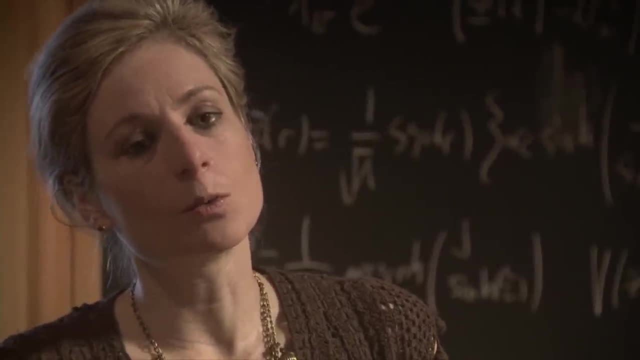 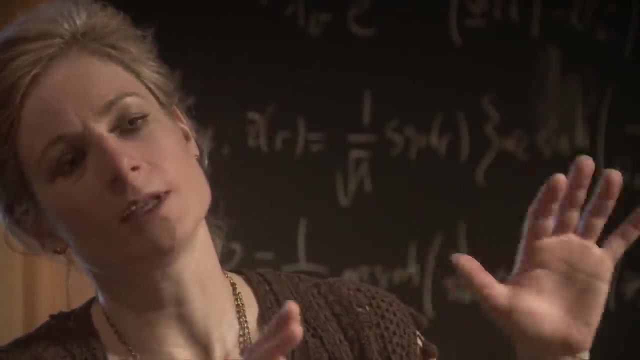 that we get away with having these forces have such different strain. So one of the ideas that my collaborator Raman Sundaram and I worked on is the idea that if space-time is really warped, it could be that gravity is essentially really concentrated elsewhere. 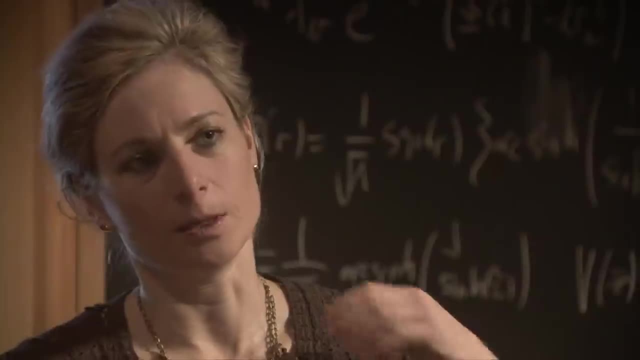 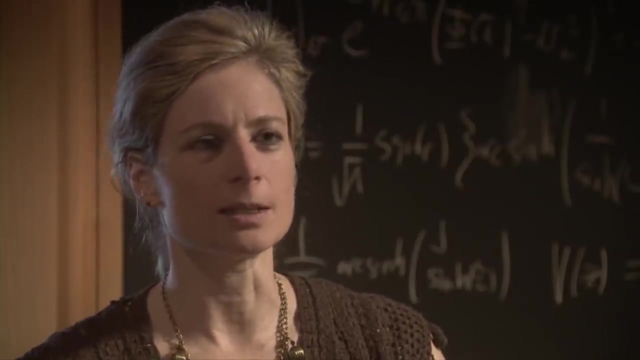 so that we are getting a very weak version of gravity where we are, So gravity could be strong, but strong elsewhere. So that's one of the things that we're trying to do. In fact, one way of thinking about it is that particles would be lighter than you expect. 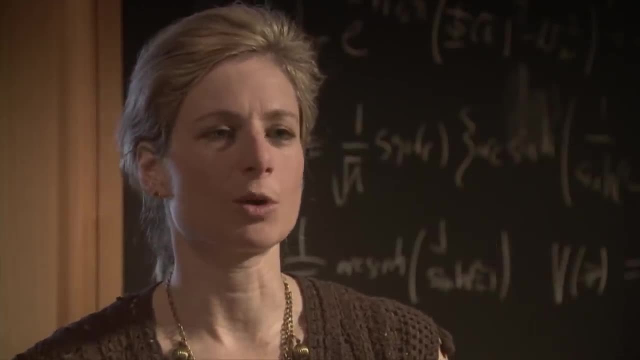 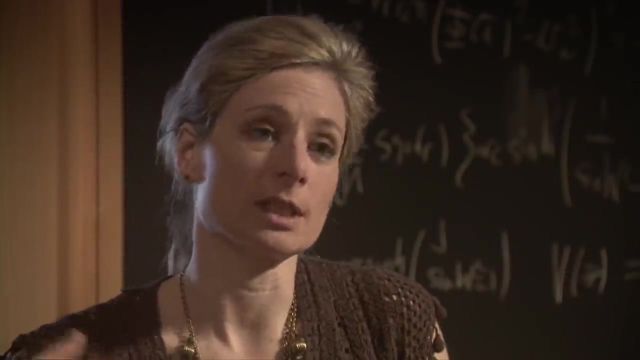 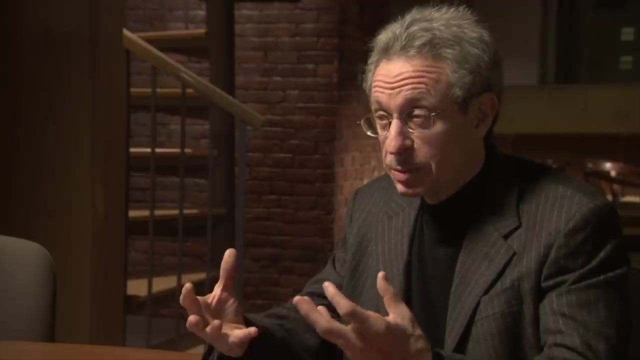 them to be in a theory without this warping. And it's because particles are lighter that you experience gravity as weaker. So this could be a very natural explanation for why we experience gravity as weak. So in that model, the primary forces of physics would be much more similar. It's just that. 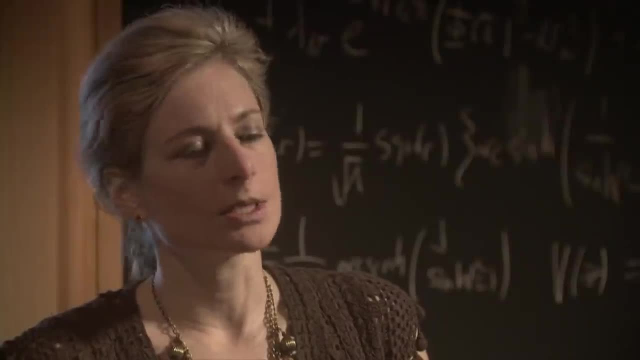 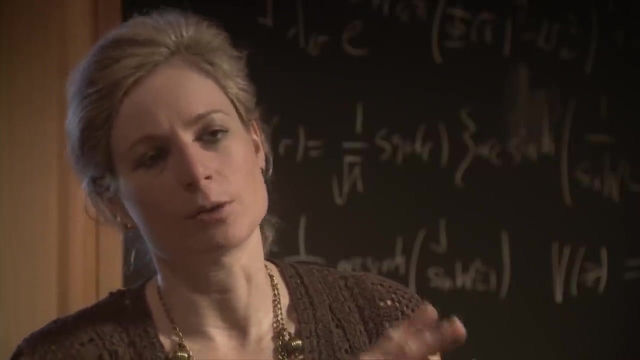 the power of gravity would be located in another dimension. Right, It has to do exactly. you can solve for it and you can see that Einstein's theory of general relativity tells you there is a particular type of warping that tells you how you experience gravity in different regions of space.